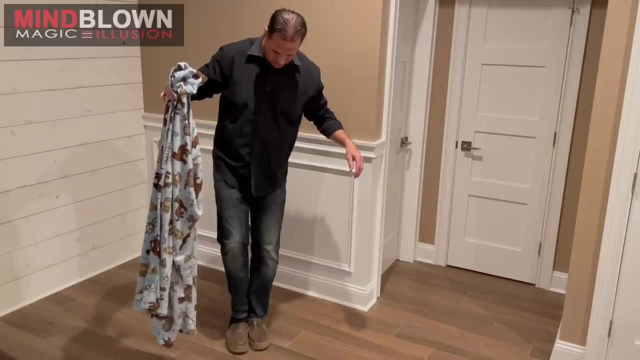 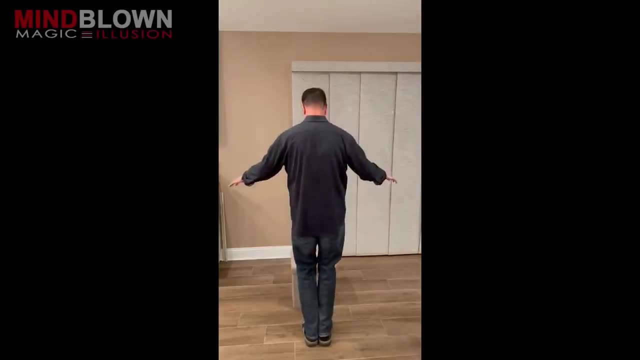 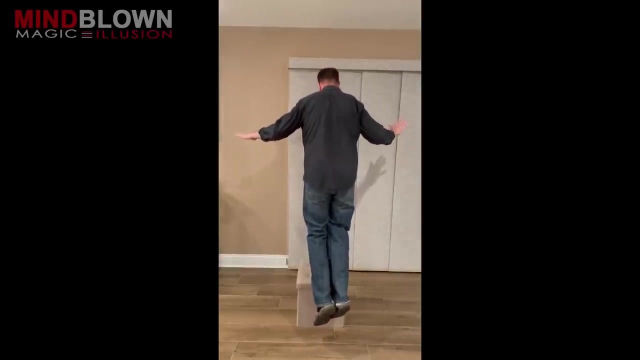 To complete this illusion, the magician puts their foot back in the other shoe and removes the blanket In this next method, with no cover at all, the magician walks up to a step stool and seems to levitate right up to the top of it. He then floats in mid-air with no visible support. 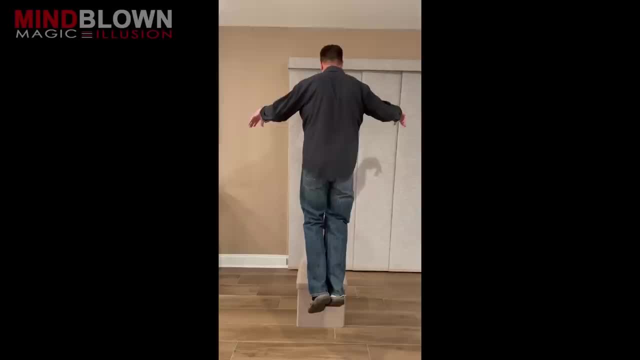 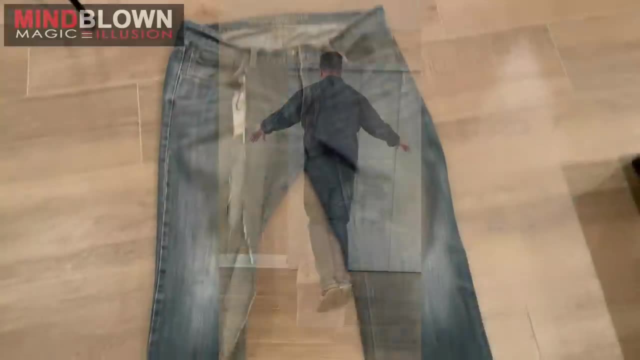 And what's great about this method is that it's very inexpensive to make and can be done at home right now. To do this, you'll need a baggy pair of pants- I like to use jeans- and then cut a slit from top to bottom on the right leg. 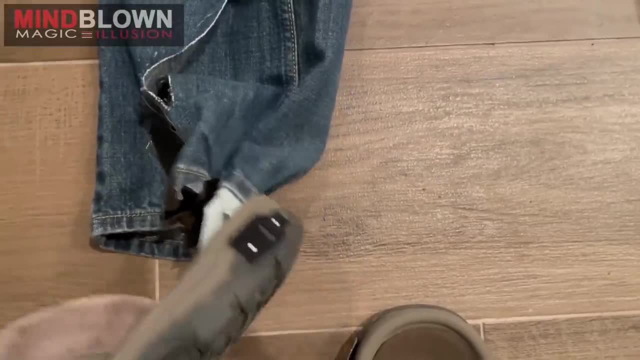 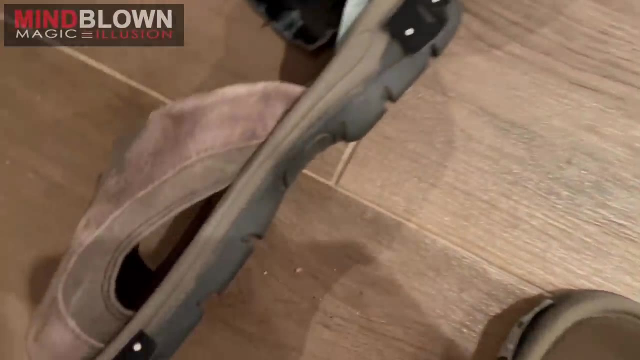 Then, from inside the pants, glue or tape the pants to the bottom of the shoe. It looks messy from the front, but remember, they'll never see this side. they see everything from the back. Next, you'll apply velcro to the inside edge of both of the shoes, or in this case I'm using sandals. The 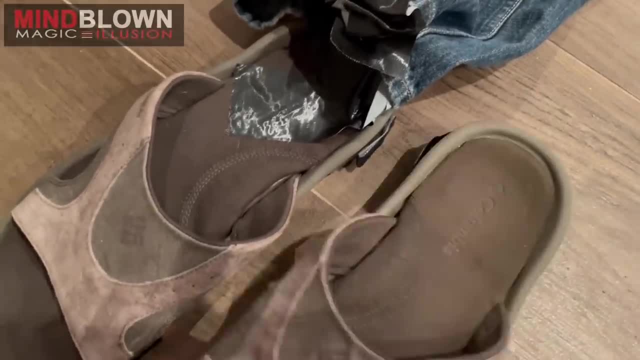 velcro is used to secure the shoe to the bottom of the shoe. If you want to use velcro to secure the shoe to the bottom of the shoe, you'll want to use velcro to secure the shoe so that when you push the two shoes or sandals together they stick to each other and when you lift one the other one. 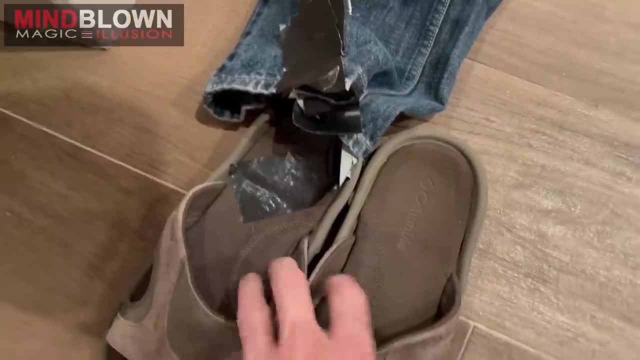 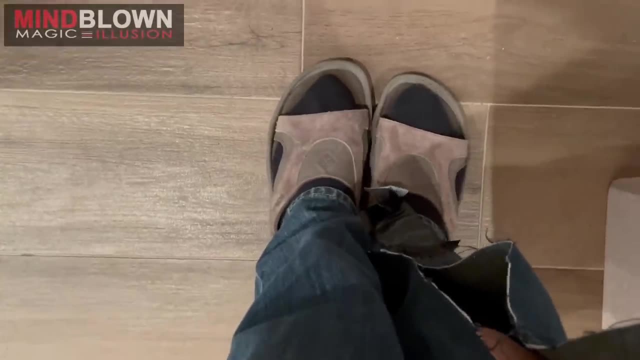 lifts as well, Very similar to what I did earlier with the rubber bands. Now, as you step up to position, you'll hold your two feet together, so the velcro sticks. This will allow you to remove your right foot from the shoe and slip your leg out of the slit inside the jeans. Now your right foot. 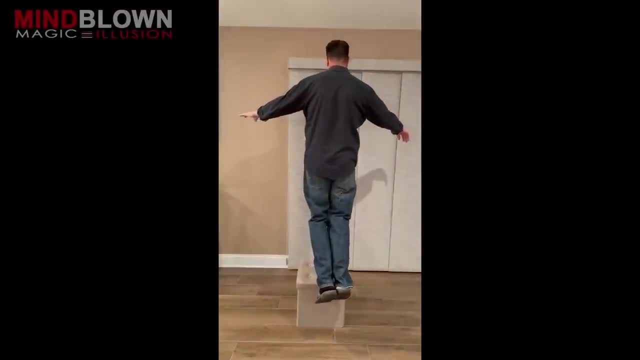 will step up onto the stool and you'll lift your body up, but from the back, the two legs stick together and it looks as though you're floating. Now you'll lift your body up, but from the back, the two legs stick together and it looks as though you're floating. 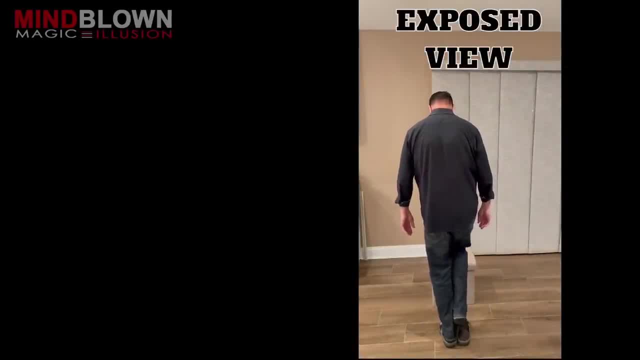 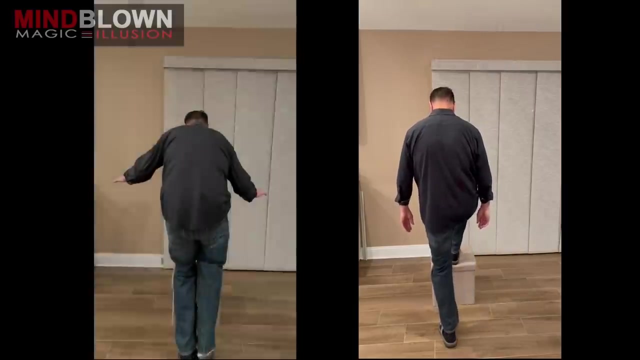 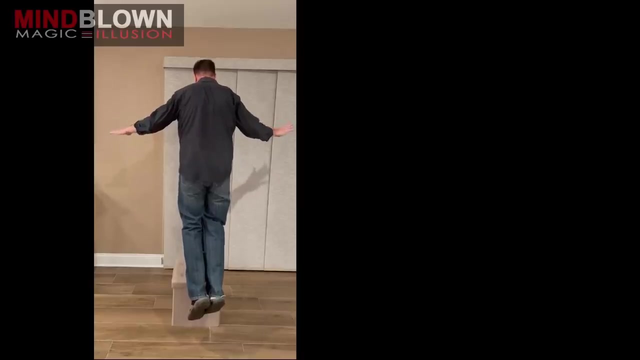 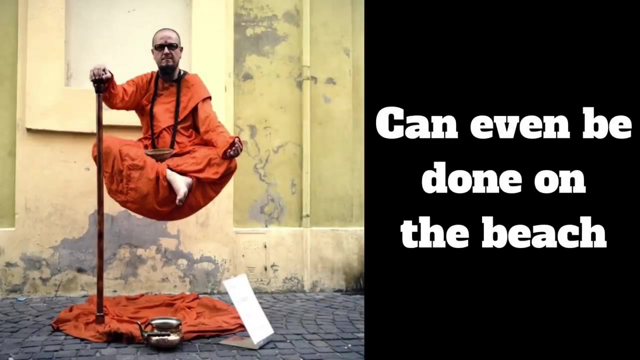 Now you'll lift your body up, but from the back, the two legs stick together and it looks as though you're floating. This next method is very popular with street performers Because there are no angles that it doesn't work from. it looks great from all around. 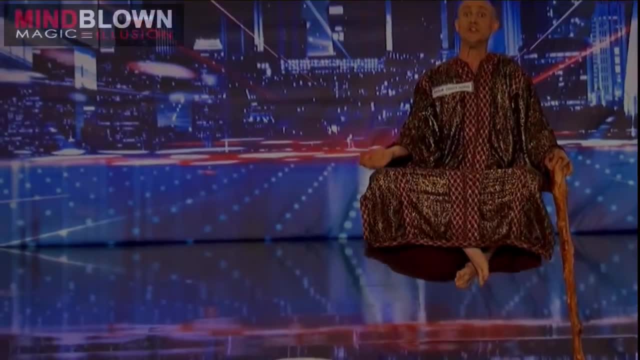 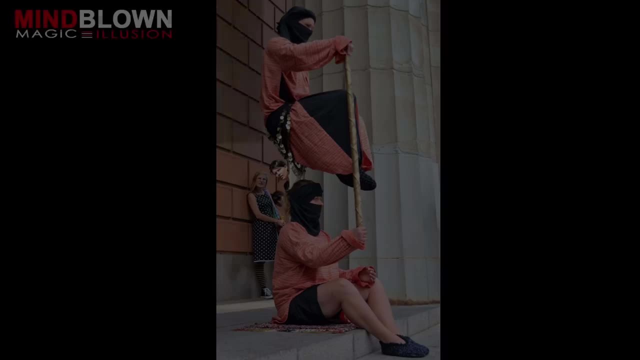 You might have even seen it on a popular television show. You might have even seen two performers doing this act together, but regardless, the method is always the same. You'll notice that in every scenario there is something on the floor, whether it's a blanket.